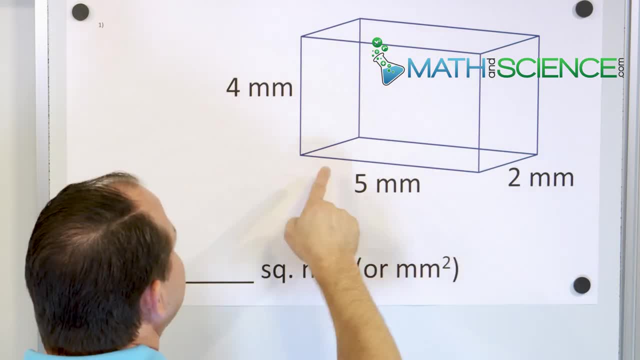 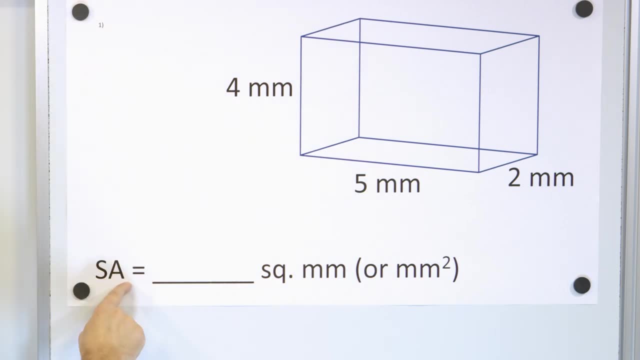 easier just to see with a picture, And I draw this as a wireframe just so you can see kind of behind it and kind of like see all of the, all the faces there. So when we want to find the surface area, we call it SA. surface area. It's the same thing as area, it's just the area of all of the. 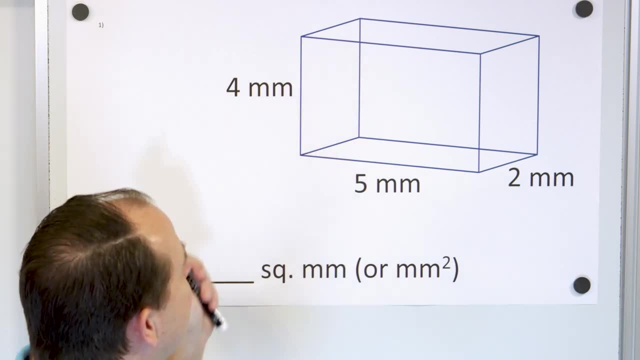 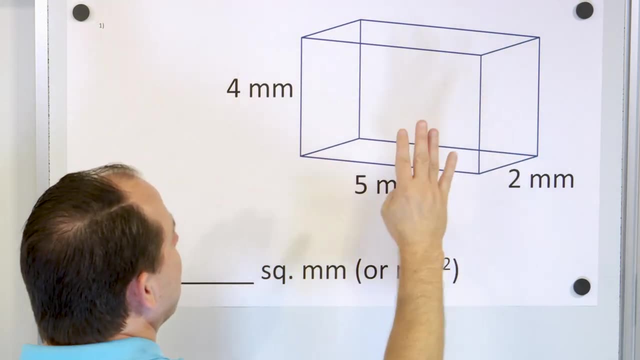 faces on all of the sides. So you can see that there are six sides to all of these rectangular solids. there's the top side and the bottom side, that's two. there's the left and the right side, that's four. And then there's the front and then the back, that's six. So there's always going to. 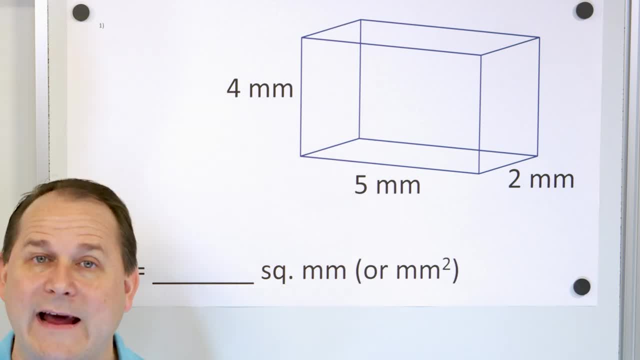 be six sides, And so every one of those sides is rectangular. right, you can see that every side is rectangular. So, really, in order to find the volume, I'm sorry, the surface area of a rectangular solid, we need to find the area of this face and add it up to the area of this face. 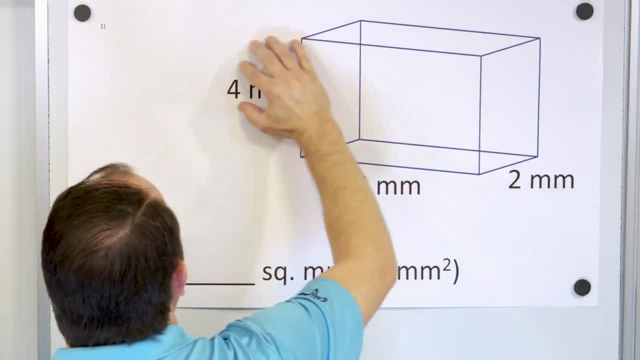 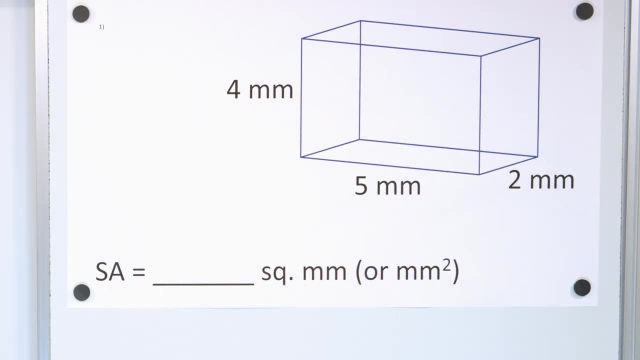 and add it to the area of this one and this one and this one and this one. there's six of them, So we're going to find kind of the area six times, sort of, and add them all together. That's the total surface area. Now we'll make it a little bit easier by drawing a picture I'll show you. 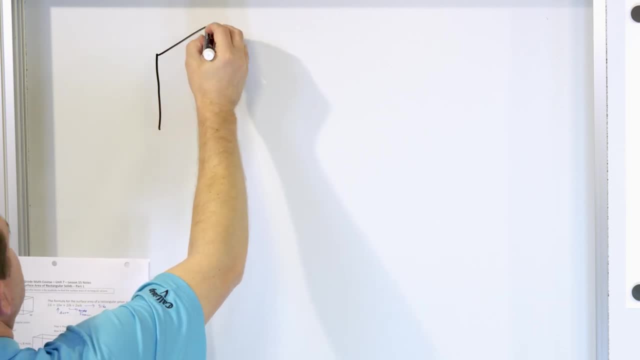 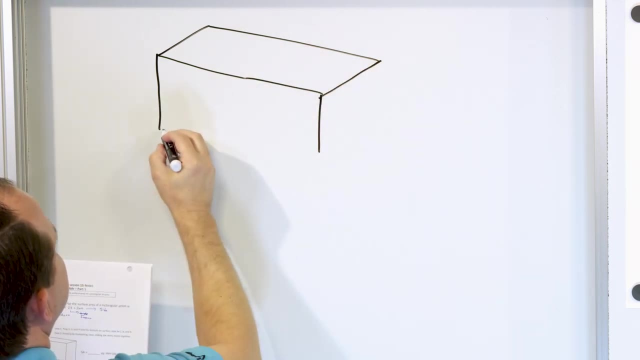 the equation that you'll see a lot of times in your book And we'll go from there. So let's just kind of try and see if I can draw this guy first. Something like this, something down here, like this, something like this. So this is a rectangular. 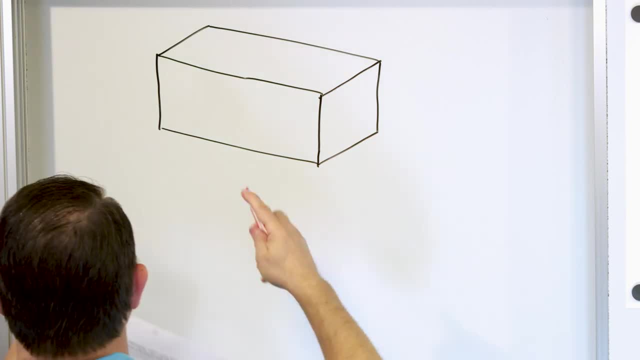 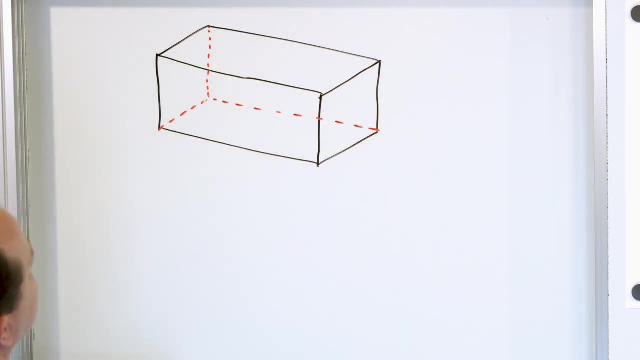 solid right, And then I can go behind here And I can say, all right, I'm going to drop this dotted line down here, something like this, something like this, Okay, so, trying to do a little, my best to do a sort of a three dimensional figure Now: length, width and height doesn't. 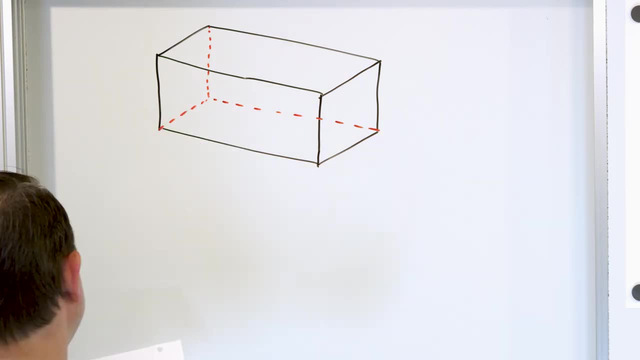 really matter because it's you can flip it around and redefine whatever you want, But typically most people would say that this direction is the height, that's how far up it is. The length is typically most people are going to say the long direction and 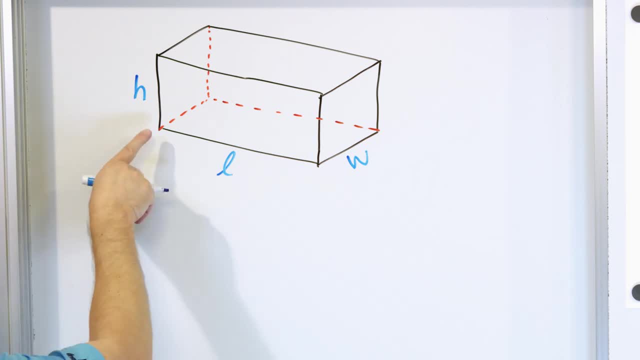 the width is going to be whatever's left over the other direction here. So there's three dimensions, there's this way, there's this way which forms a rectangle on the bottom. And then the height of the thing is just how far the thing is sticking up. Now, if we were to find the surface, 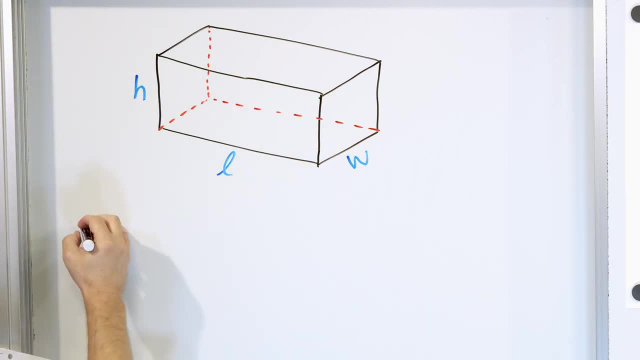 area of this. how would you do it Right? How would you do it? Well, what you would say, we'd call it surface area, to say that we're finding the area over all of the surfaces. What you would say is the area of the bottom right. So the bottom is a face right here, but it's, it forms a rectangle And 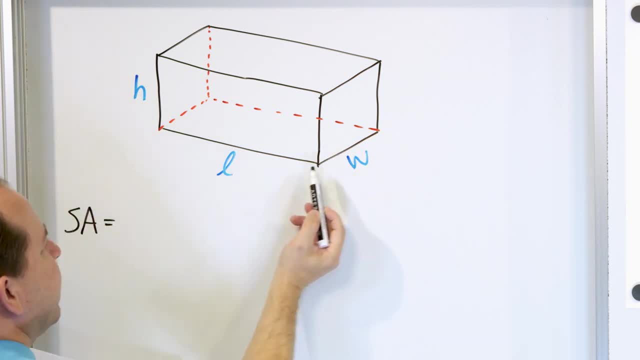 one direction of that rectangle is L and the other direction is W- length and width. So we know that it's going to be L times W, right? That's the area of this bottom one here, right? But there's two of those And the area of the top one also has the same dimensions, because this is also L and this. 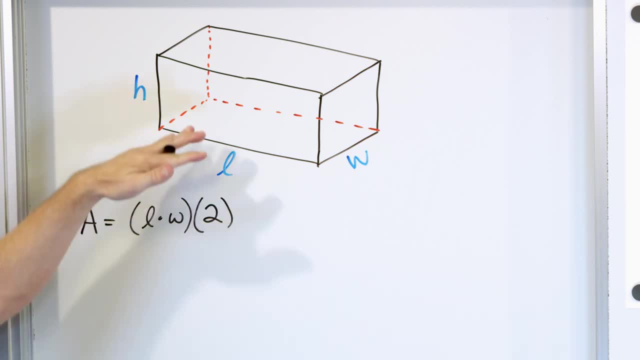 is also W. So we'll just multiply that by two. So we find the area of the bottom, and then we double it, because the area of the top has exactly the same dimensions. So that's what this looks like, But then we have to add to that the area of the other faces. So let's look at the front and 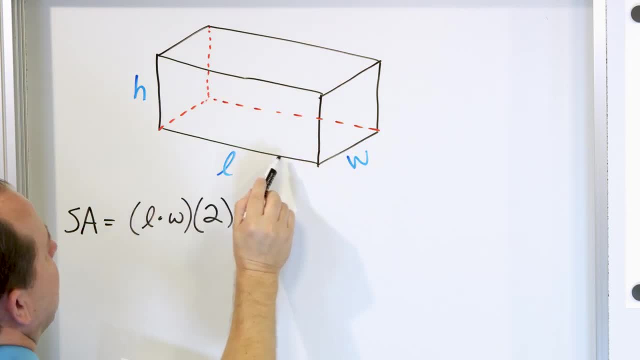 the back, this face and the one here. It has a dimension of L and also a height of H, right Of LH. So it'll be the length times, whatever the height is, That will give me the area of the face that's on the front here. L times H, but I have two of them also, So I multiply by two because I 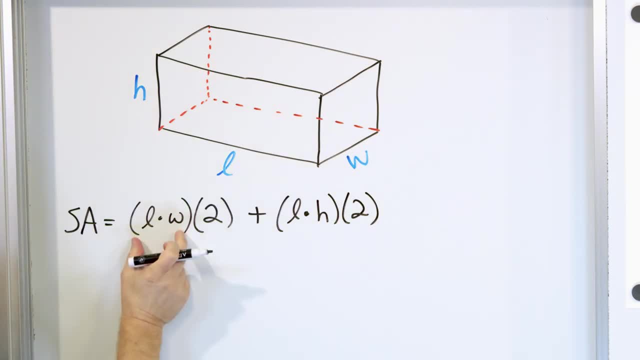 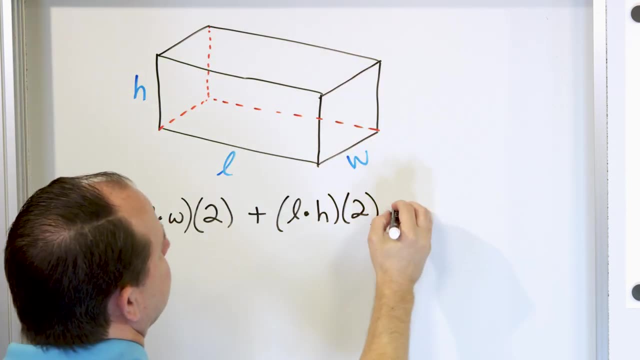 have a top and I also have the one on the back. So I'm finding the area of the bottom. multiply by two because I have a top, I have the area of the front, but I multiply by two because I have the back right. And then what is the other area? It's the sides here, right. So it's W is the dimension. 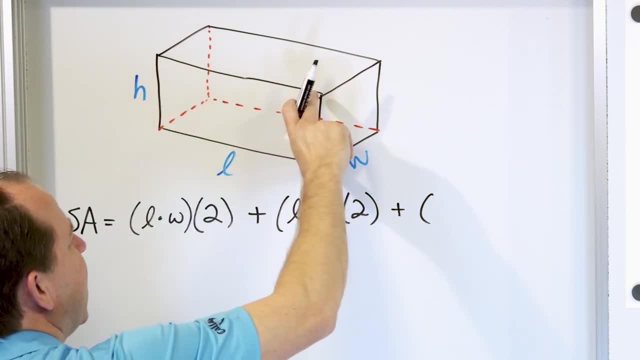 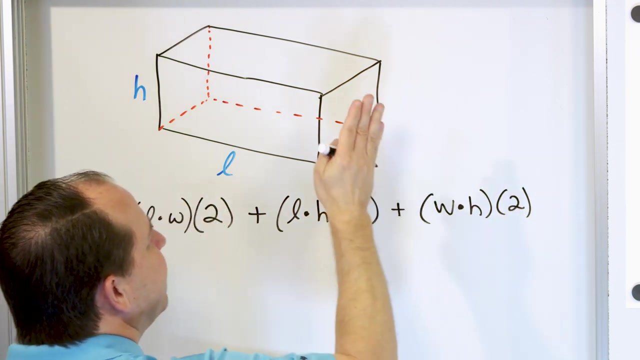 here. And then I have height, but don't forget, this is also the height down here as well. So this is the height, and then W forms the two dimensions of the side rectangle there, So it's HW, so I can call it W times H. And then I multiply that one by two, because I have one area here and 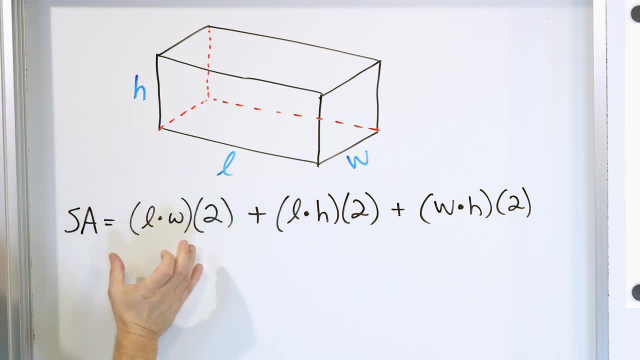 then one on the other side. So from the top for the bottom, I have this area, the bottom L times the length times the width, but I'm doubling it because I also have a top. And then for the front, I have the area length times height right here, but I'm doubling it because I have a back face. 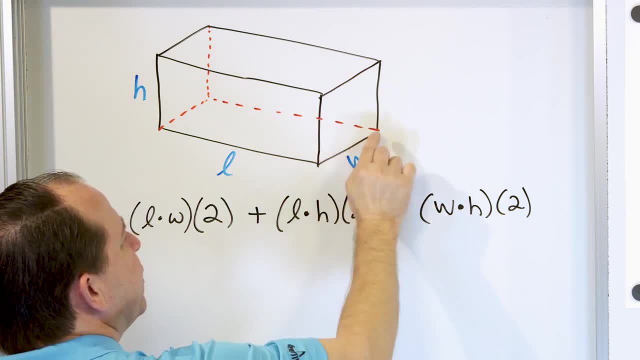 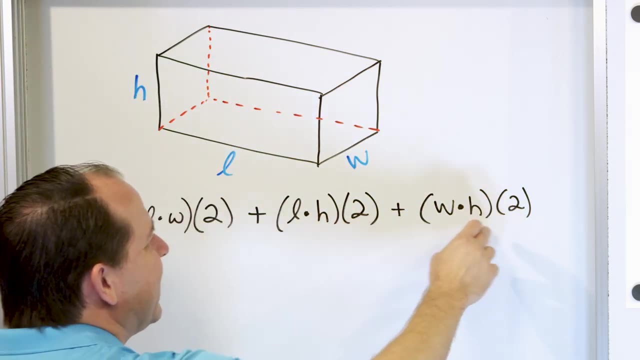 which is the same size, And then for the right-hand side it's W times H. That's the area of this, but I double it because I have the other side. So I have two sides, four sides, six sides altogether. 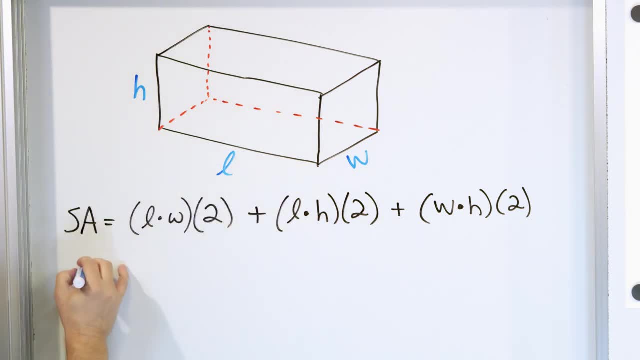 And that's what this equation is Now typically what you'll see, the way you'll see it written like in a book or something like this, is: you'll see it as 2LW plus 2LH plus 2WH. Some of the 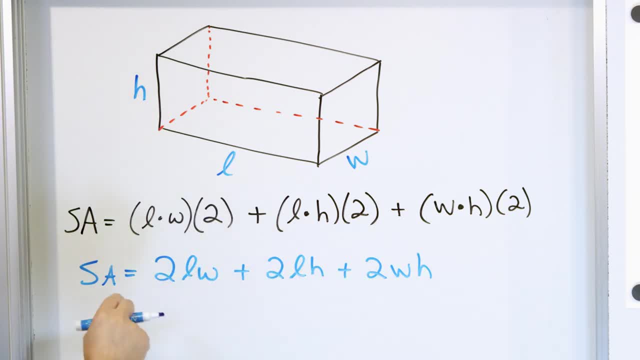 letters might be flipped around, but you get the idea. Let me double check: 2LW, 2LH, 2WH. Yeah, that's right. So you can use this equation. You know, students you know say: Hey, this is the surface area of a rectangular prism And 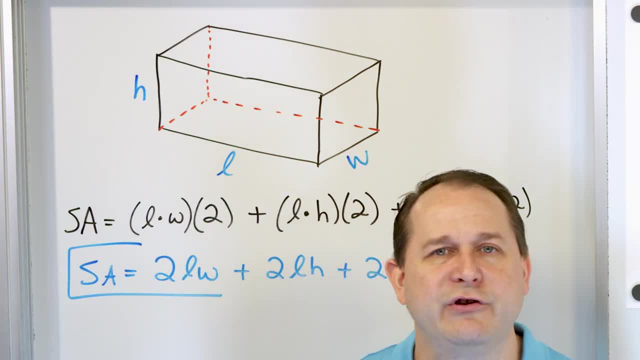 they'll just memorize it. But the problem is is that it gets confusing to use that formula- Which one is L, Which one is H? And then you start just trying to put things into it. You know, put the proper things in the proper locations. You don't really often know what you're doing. 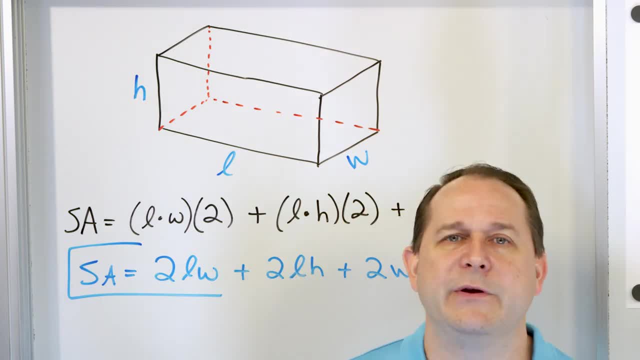 You're just trying to put the numbers in the right spot and calculate, but you often make mistakes because there's so many letters. So I'm showing you this because I want you to understand exactly why the twos are here. we talked about that. 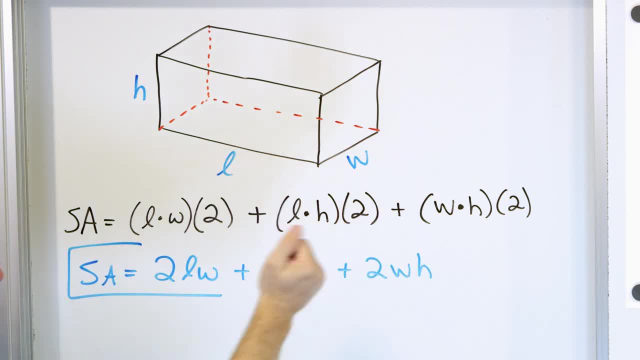 why the letters are here. we talked about that, but I'm actually not gonna use this equation at all when we actually calculate. So you'll see what we do here in a minute, But this is the idea of what you'll see in a book. 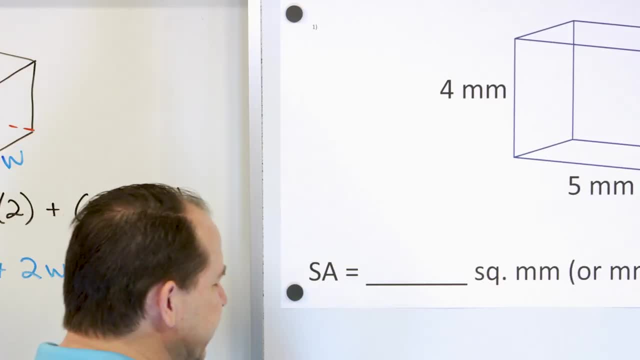 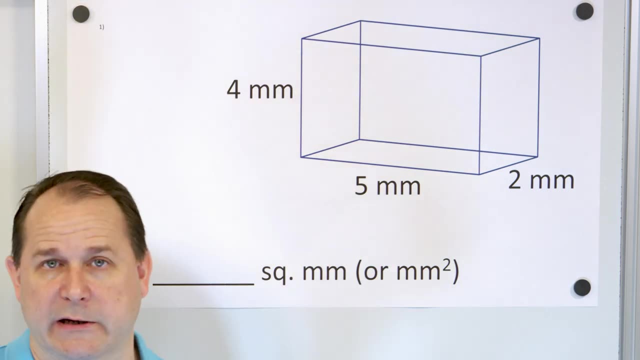 and why. you will be told that this is the surface area. So let's go over here and actually solve our first problem. What I'm gonna do is forget about the formula. Sometimes students just plug into a formula and sometimes the formula gets in the way. 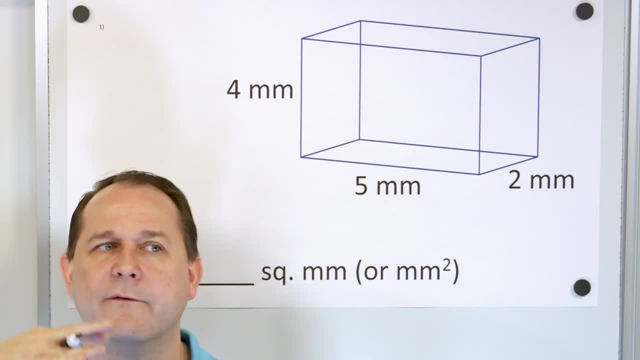 It's better for you to understand what you're doing. You're trying to find the area of all the faces, But since it's a rectangular prism, the top and the bottom are always the same. the left and the right are always the same. 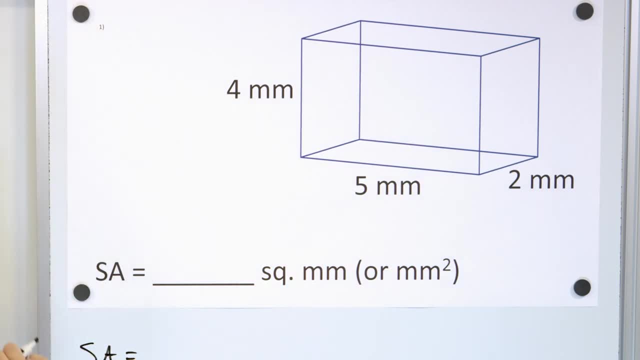 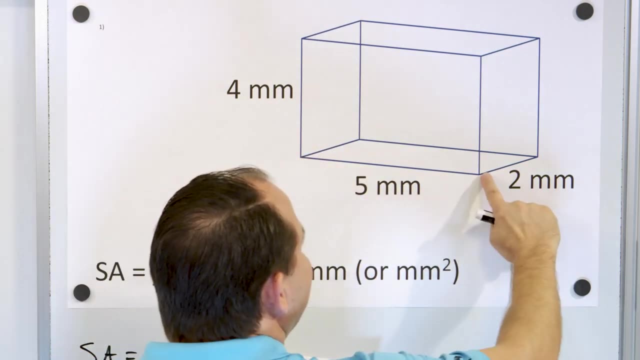 and the front and the back are always the same as well. So instead of trying to plug it into a formula, let's just look at the bottom here. The bottom of this thing is five millimeters long and two millimeters deep, So I can find the area of the bottom. it's five times two. 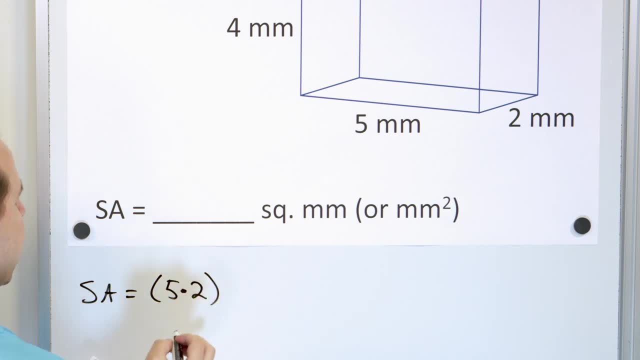 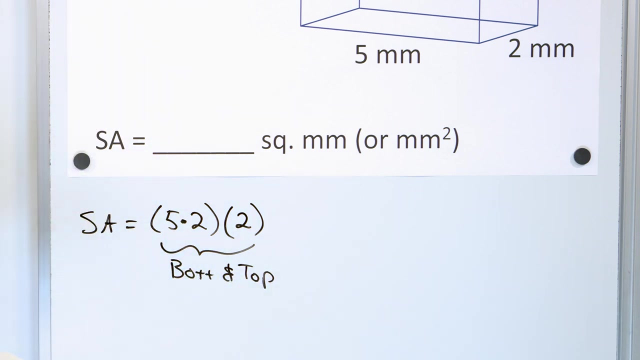 So the area of the bottom is five times two. But I have two of those because I have an area on the bottom and on the top. So I multiply by two. So this little calculation is bottom and top. So bot means bottom and top right. 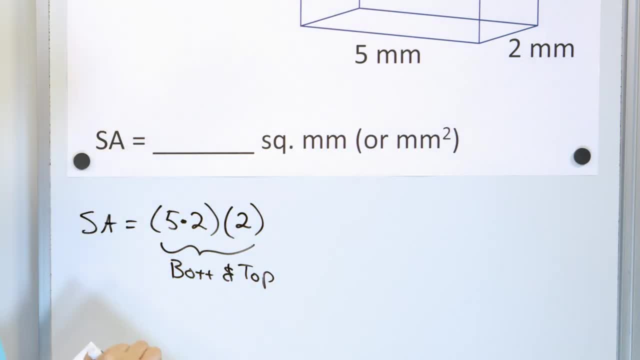 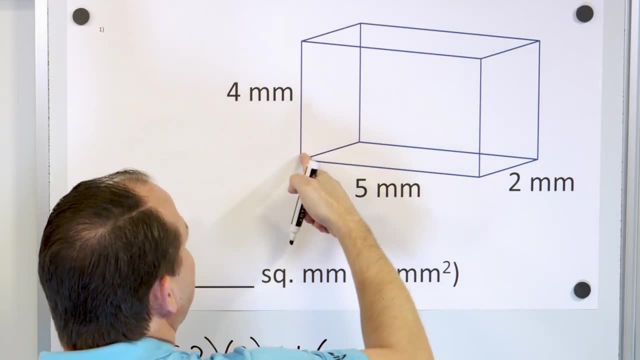 So I have five times two for the area, but I multiply by two because I also have a top and I have to add to that something else. So let's take a look at the front. The front is four millimeters tall and five millimeters wide. 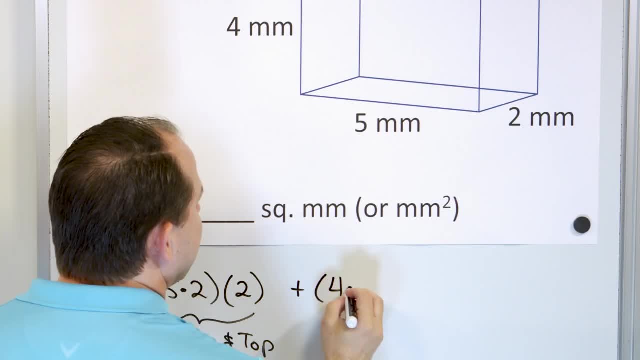 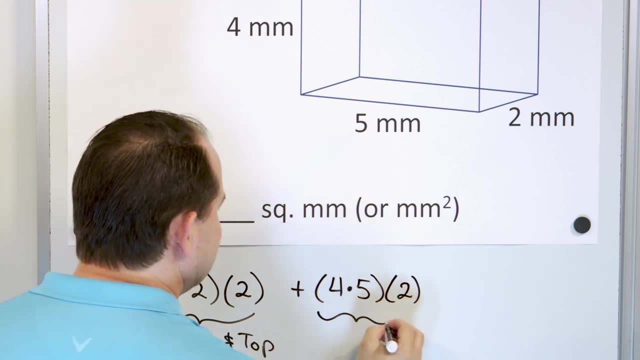 So five times four, or four times five, So put four times five. that's the area of this front, that's the area of the face, but I have two of them, So I multiply that by two And this is front and back, like this: 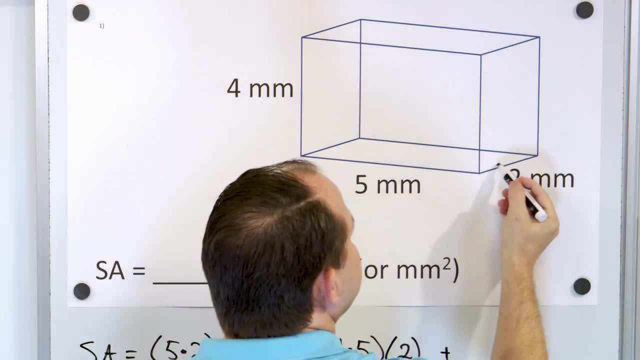 And then I have the area of the side. So let's take a look at this side. It's two millimeters this direction. The height of it is here, but it's the same as the height here, which is four. So it's two times four. 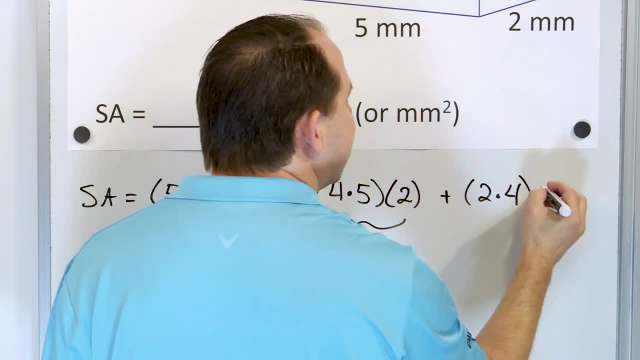 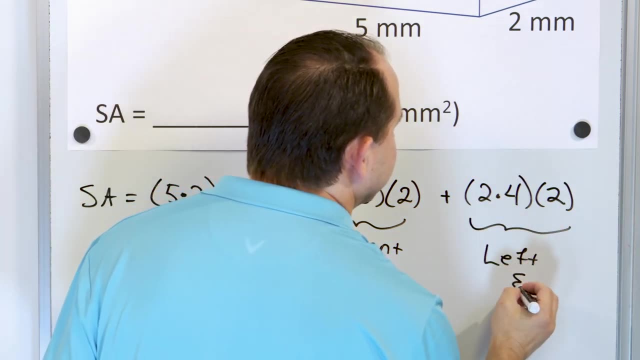 So two times four. that's the area of this side, but I'm gonna double it because I also have another side on the other side Place there. I'll call this left, and right, Right. So you see, I never really used the formula. 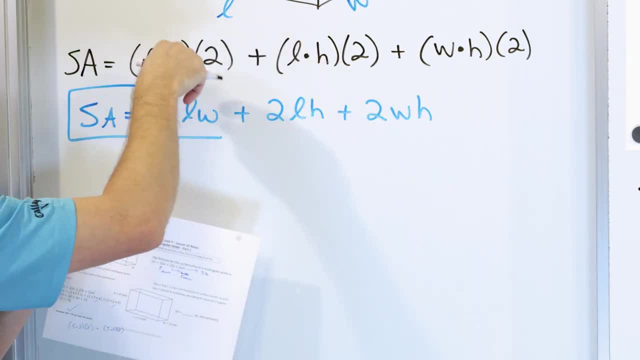 I didn't really write this equation down and say, okay, what was L put it here here, here? What is W put it here, here, here? You can do that if you want, But to me it's actually much easier. 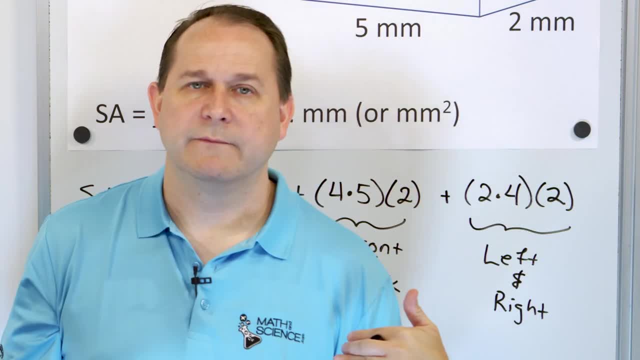 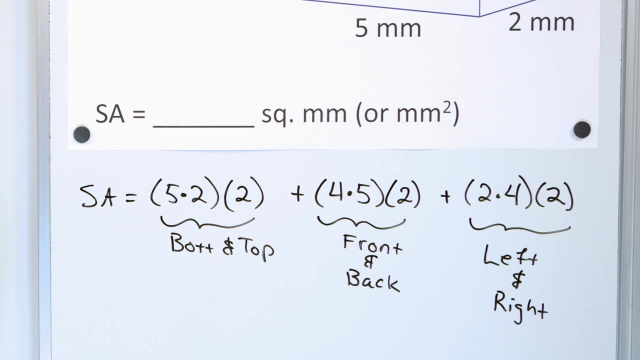 to just look at the figure: find the area of the bottom, then times two for the top, then find the area of this times two, And then I have it all written down without stressing out over where the letters go. So now we can calculate. 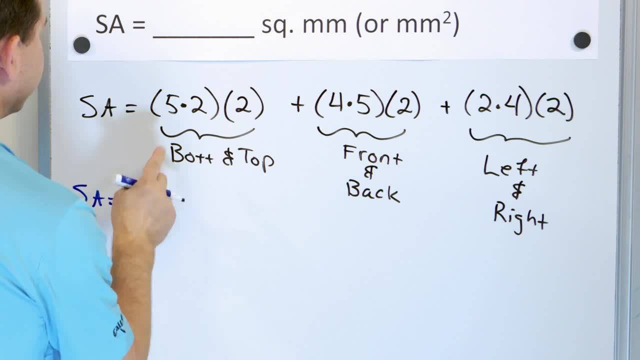 So the surface area is going to be equal to now I have 5 times 2, which is 10, I still have to multiply by 2.. Here I have 4 times 5 is 20, I still have to multiply by 2.. 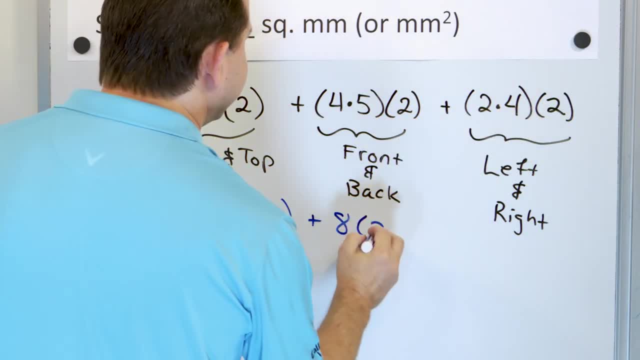 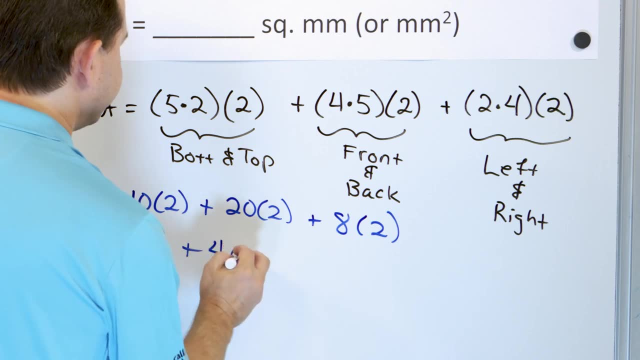 Here: 2 times 4 is 8, and I still have to multiply by 2.. What is 10 times 2?? It's 20.. What is 20 times 2?? It's 40.. What is 8 times 2?? 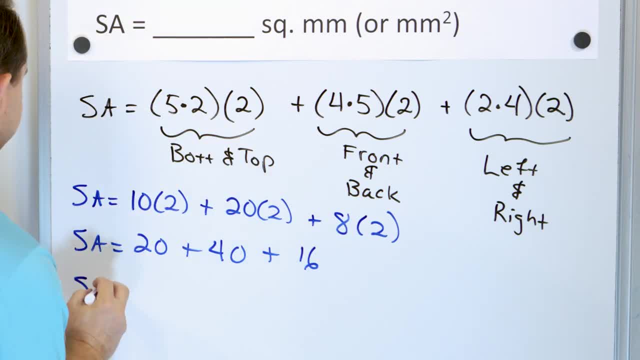 It's 16.. We can line these up and do column addition, but these are actually easy to do in our head too. 20 plus 40 has to be 60,, 2 plus 4 is 6.. So this gives us 60,, and then, going up, 10 more is 70, and then 6 more is 6.. 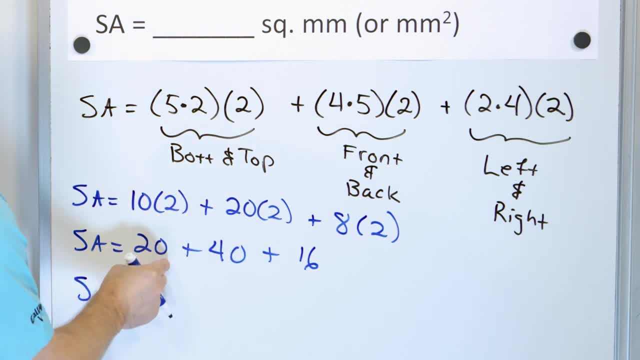 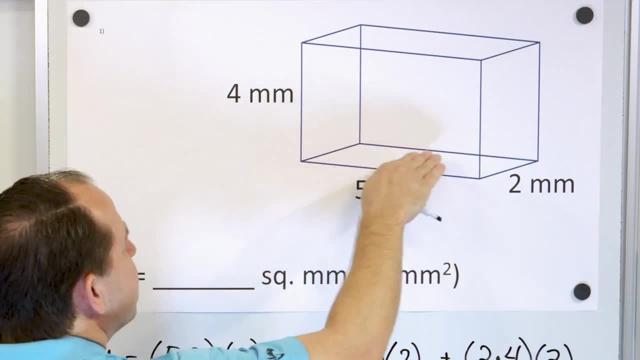 So 76.. So you have to say 40,, then 60,, then 70,, then 6.. So 76.. 76 is the answer and it is square millimeters for the bottom and the side and the top and everything is square millimeters. 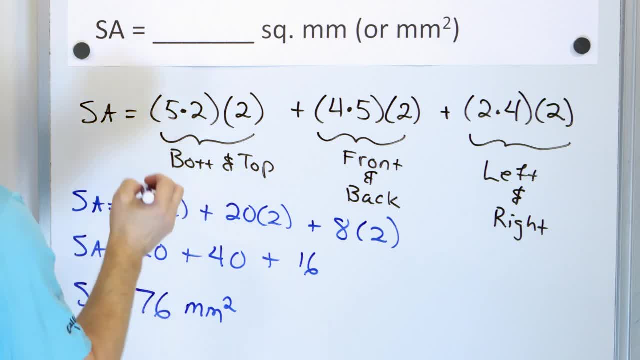 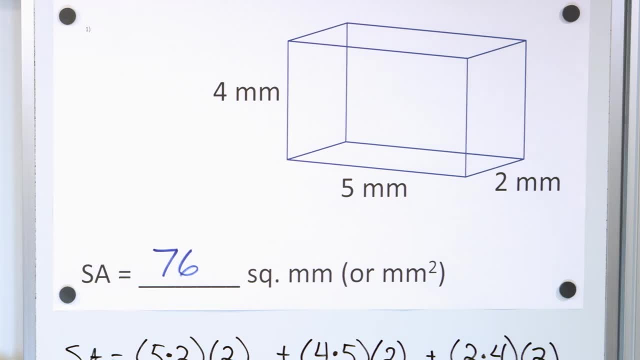 We add them all up, We still get square millimeters. So it's 76 square millimeters. Now the first example always takes the longest because you have to describe what is the equation, how does it work, what are we doing, and all that. 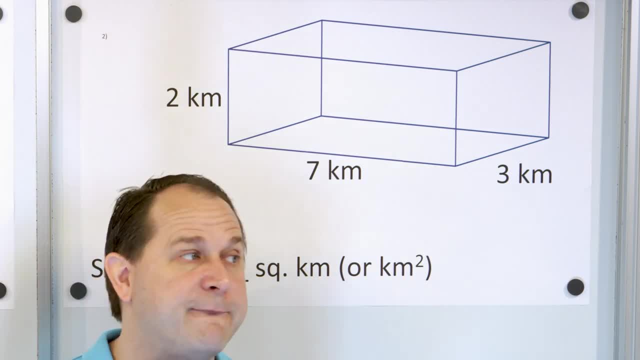 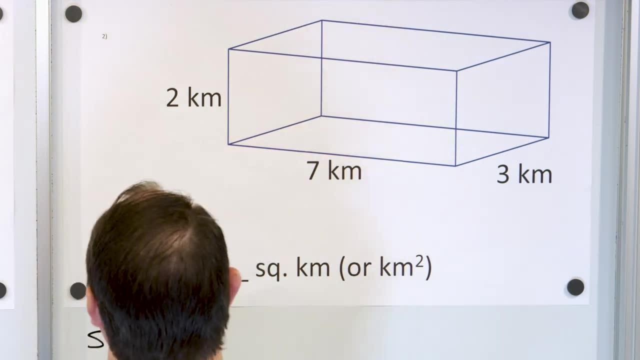 The rest of them will go a little bit faster, but that's just the same concept we're going to use for every single problem. We're just going to get a little more practice doing it here. So what is the surface area of this rectangular prism? 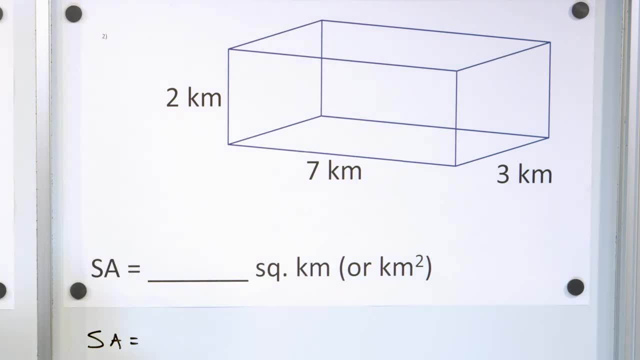 It has different units and, of course, different numbers as well. So let's first examine the bottom. The bottom is 7 in this direction and 3 in the other direction, so 7 times 3.. So I'm going to write it as 7 times 3.. 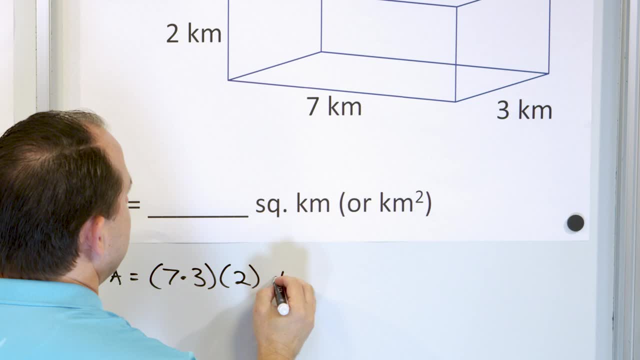 That's the area of the bottom, but I have two of those, So that's the bottom and the top. Now what's the front? The front is 7 times 2.. That's the area of the front: 7 times 2.. 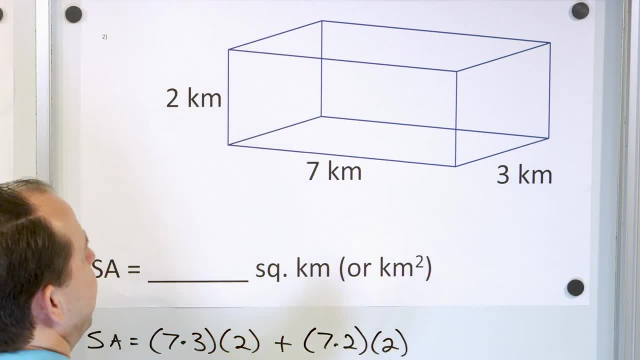 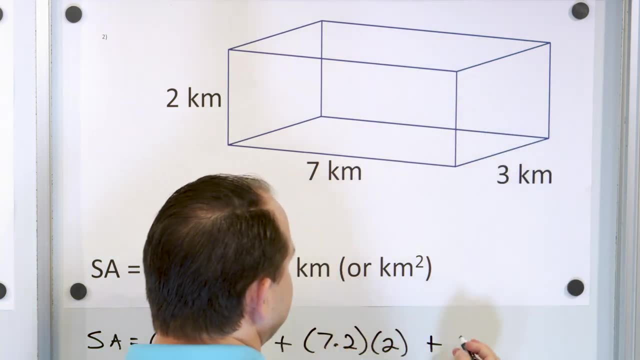 So 7 times 2, but I'm going to double that because I have a front and a back, And then the left side, or the right side, is 3 times. this dimension is also down here- 2.. 3 times 2.. 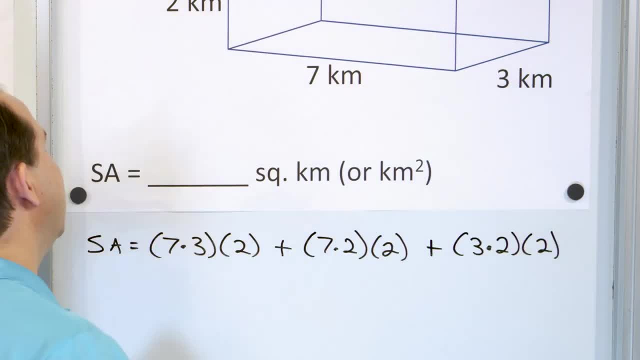 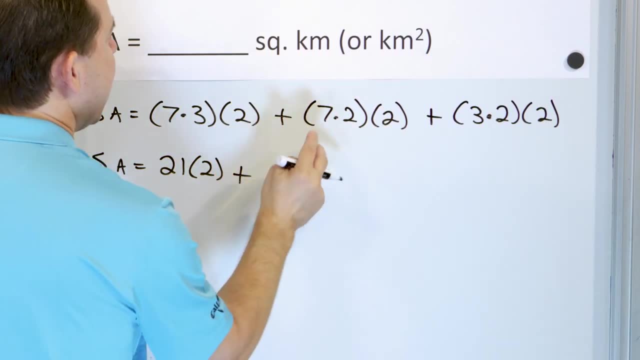 And I'm going to double that, because I have a left and a right And now I just have to carry out the multiplication: 7 times 3 is 21 times 2.. And then 7 times 2 is 14 times 2.. 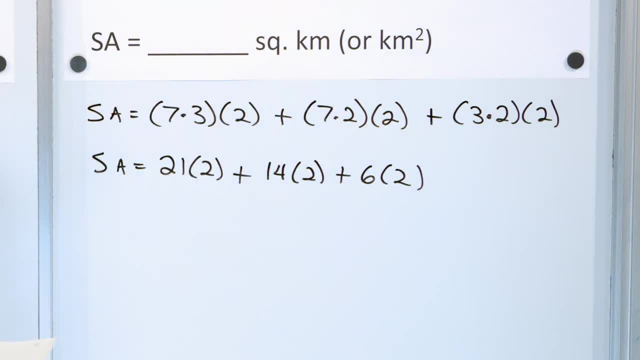 And then 3 times 2 is 6 times 2.. Now what do I have here? 21 times 2, I think you can convince yourself. if you double this and double this, you just get 42. And then 14 times 2, if you multiply that out, you'll get 28.. 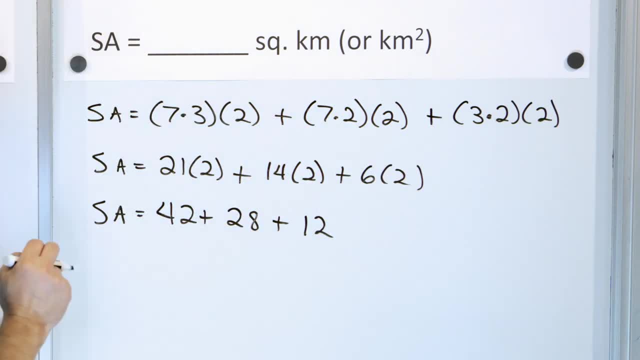 And then, if you multiply this out, you'll get 12, right? So you're going to add these up. I'm assuming you know how to add and carry by now. So when we add all three of those numbers together, we're going to get 42 plus 28 plus. 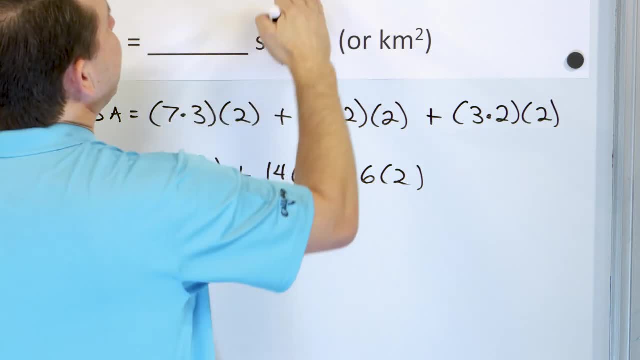 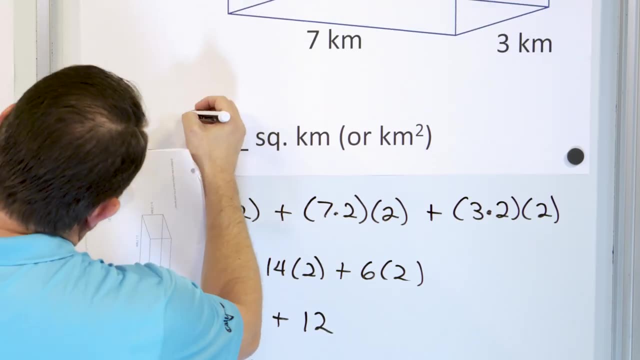 12 gives you 82 exactly, And the unit- because I had area in kilometers square kilometers everywhere- is the total area is in kilometers squared as well. So the answer is: let me just double check: 82 square kilometers. You find me checking my notes a lot because I make mistakes too right? 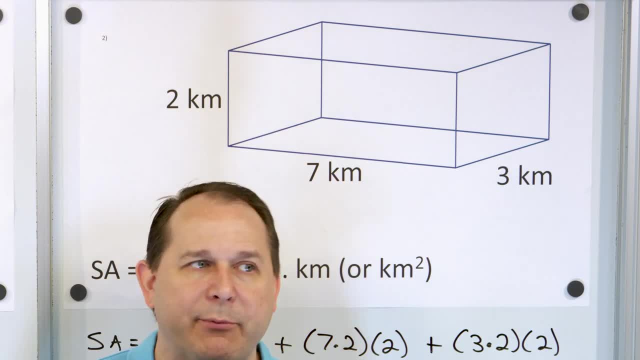 And I know that I make mistakes. I have the answer here, but I'm not copying from my paper. I'm doing the work, but I'm just double checking, making sure I haven't made a mistake, because I make mistakes all the time. 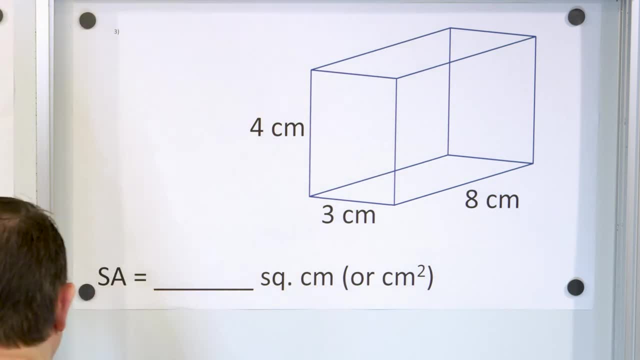 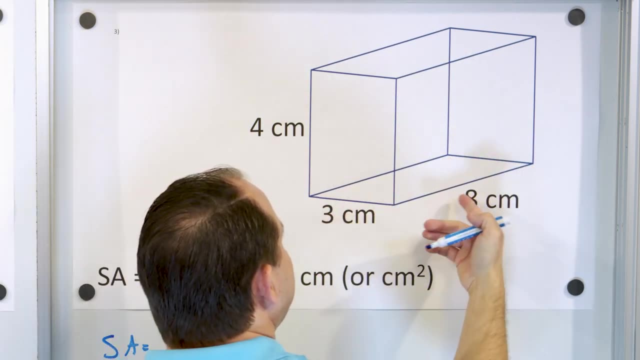 All right, here we have problem number three. Let's find the surface area of this guy right. Let's take a look at the bottom. The bottom is this face. It's 3 times 8.. That's going to give us the area of the bottom right. 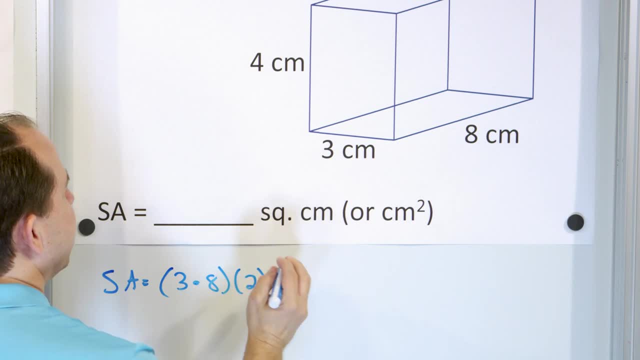 3 times 8.. But I have two of those, for the bottom and the top, so I'll multiply times 2, right? What about the front and the back? This is the front. This is the front. Let's call that the back. 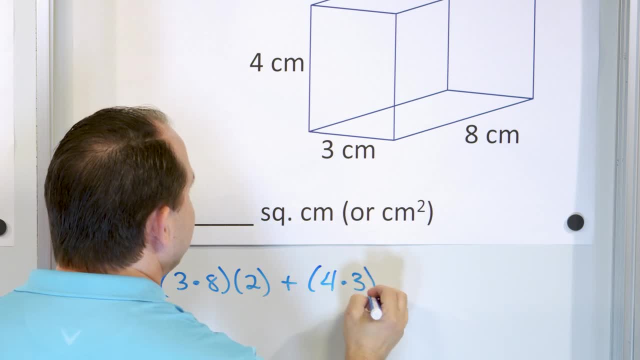 4 times 3 would be the area of the front- 4 times 3.. But I have two of those, so I'll multiply by 2.. And then the side- Here's the side, It's 8.. And then here we have 4.. 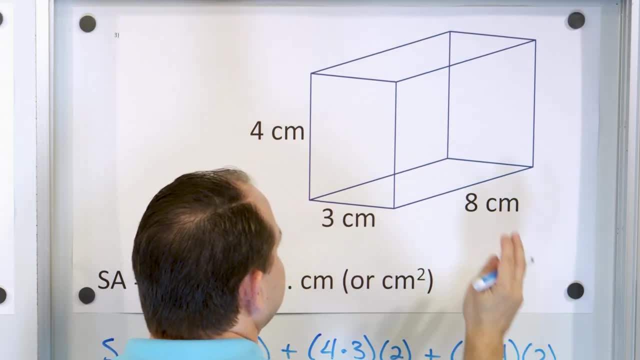 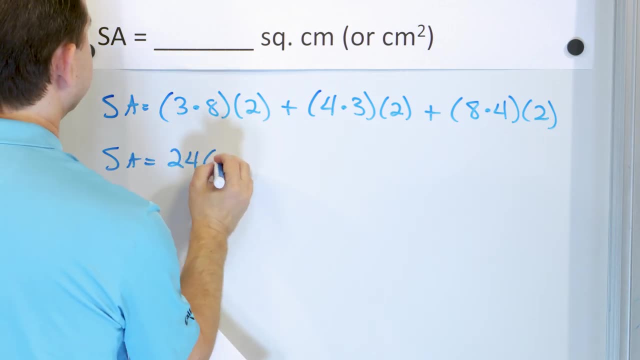 8 times 4 is the area of the side, but I have two of those, So I have 8 times 4, and I have another one. So what do I have? 3 times 8,, 24 times 2.. 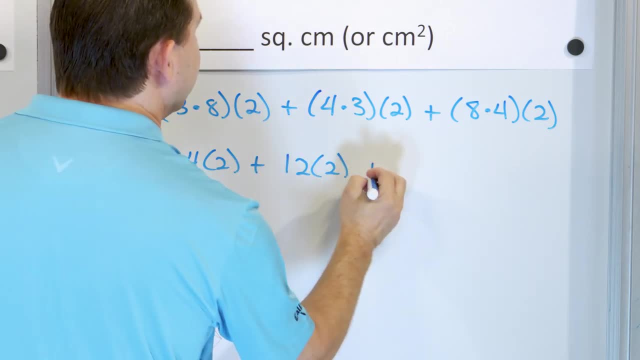 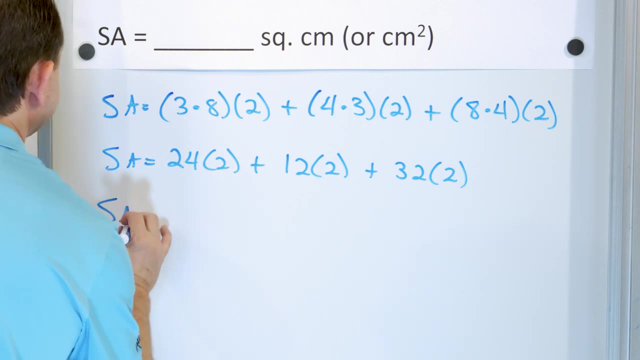 And then 4 times 3 is 12 times 2.. And then 8 times 4 is 32 times 2.. Let me just double check myself. All right, let's take a look. What do we get when we multiply 24 times 2?? 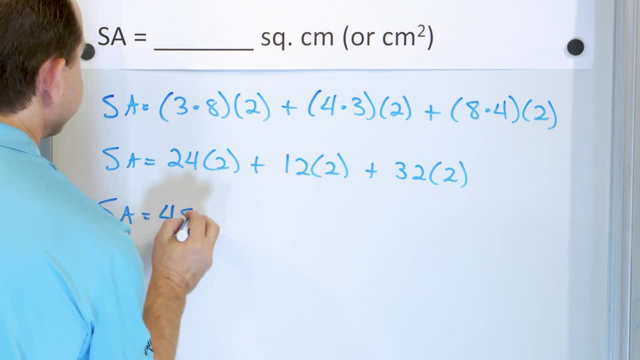 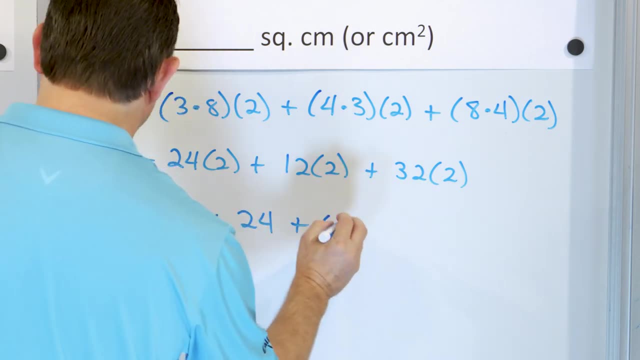 If you double each of these- I think you can convince yourself- you'll get 48.. 12 times 2 is 24.. And again, if you double both of these, you'll get 64.. So let me just double check: 48 plus 24 plus 64.. 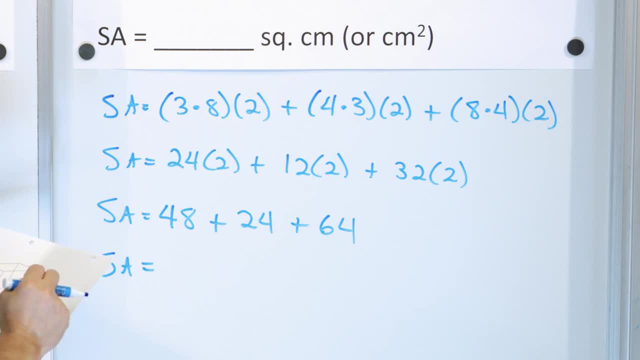 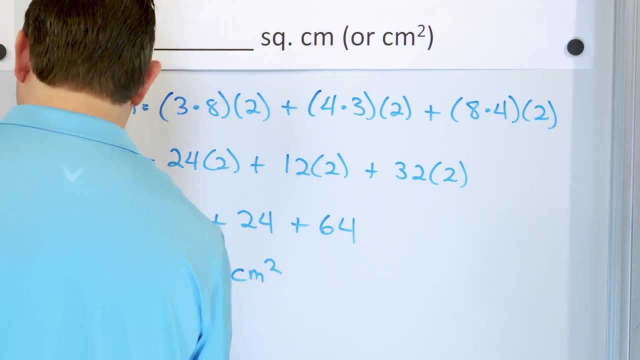 If you line these up and add them, I'm convinced that by now you know how to add. you'll get 136.. And the units? Because it was in centimeters. everywhere is centimeter squared or square centimeters. 136 square centimeters. 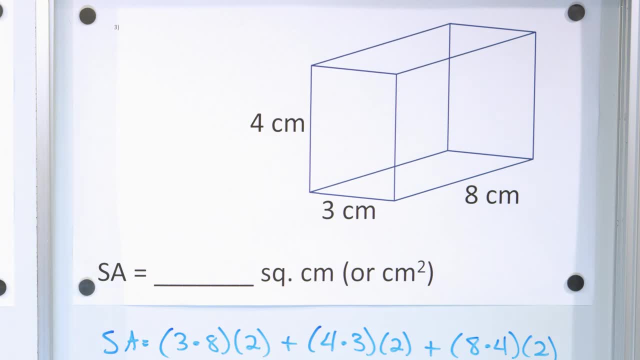 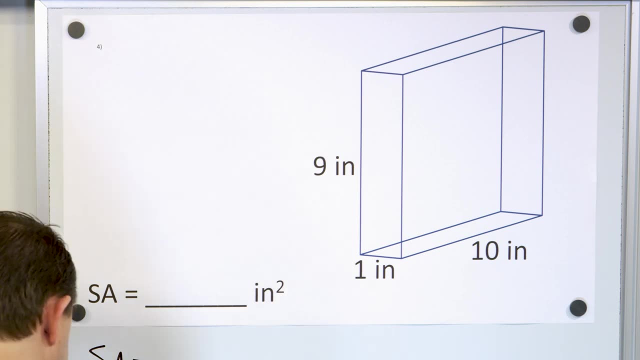 I do have one more. Let me take these down and we'll conquer our last one right now. All right, here is our very last problem. Let's calculate the surface area of this rectangular prism. So let's take a look at the bottom right. 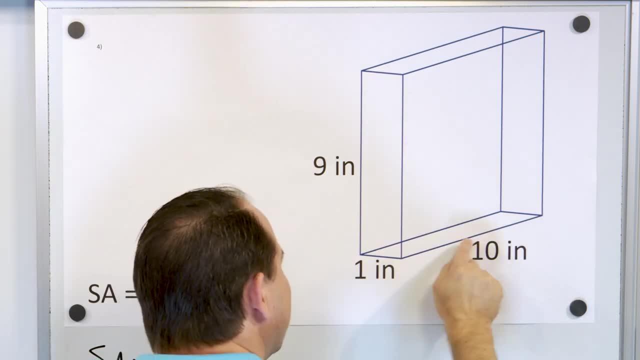 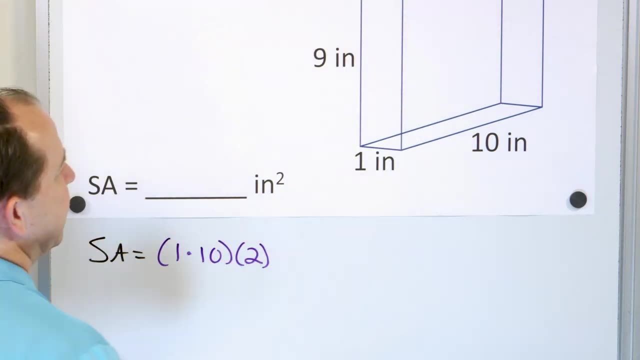 We have 1 inch in one dimension and 10 in the other, So 1 times 10 is the area, So call it 1 times 10.. And I have two faces, The bottom face and the top face. So that's the area of the top and the bottom. 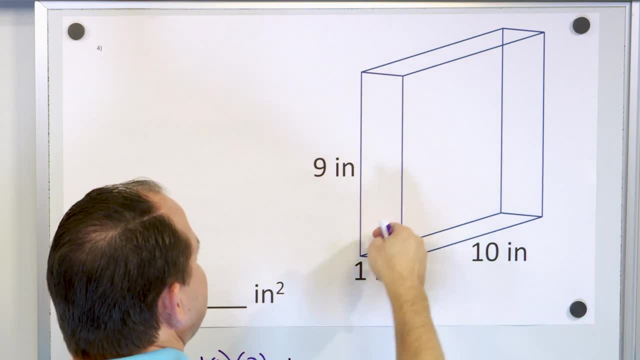 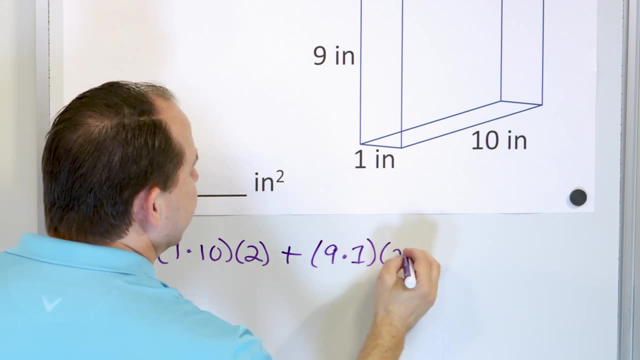 And then for the, let's take a look at the front and the back. The front would be this little bitty face here, 9 times 1.. That's the area there, 9 times 1.. But I have two of those faces, because I have the front and I also have the back right there. 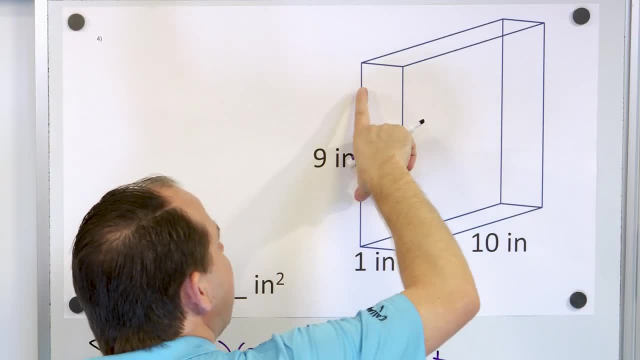 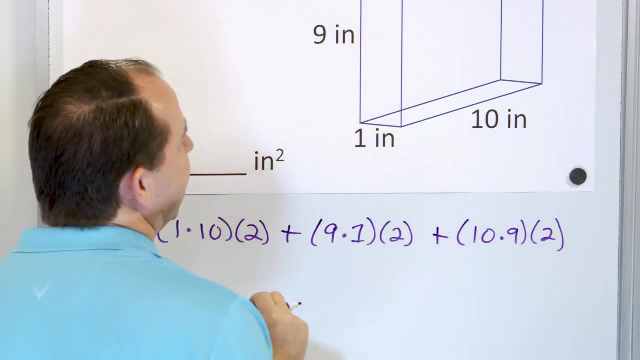 And then I have the right and the left side. Now the right side is 10, and the 9 dimension is the same here, So 10 times 9, but I have two faces there, So it's the right and the left there. 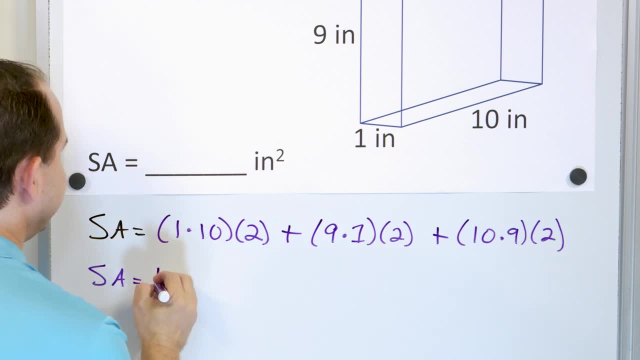 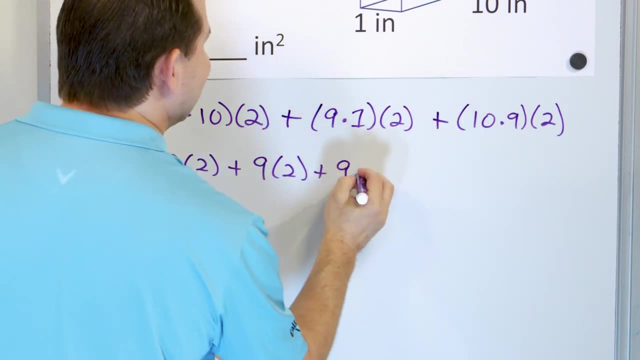 So. So let's go ahead and continue calculating. Here we have: 1 times 10 is 10 times 2.. 9 times 1 is 9 times 2.. 10 times 9 is 90 times 2.. And so what do I get? 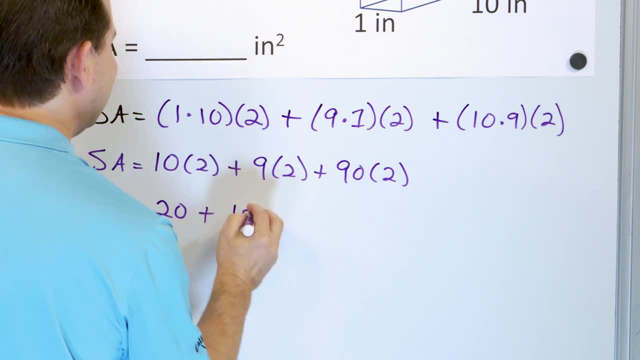 10 times 2 is 20.. 9 times 2 is 18.. And 90 times 2 is 180, because 9 times 2 is 18 with another 0 is 180, right? So what is the surface area? 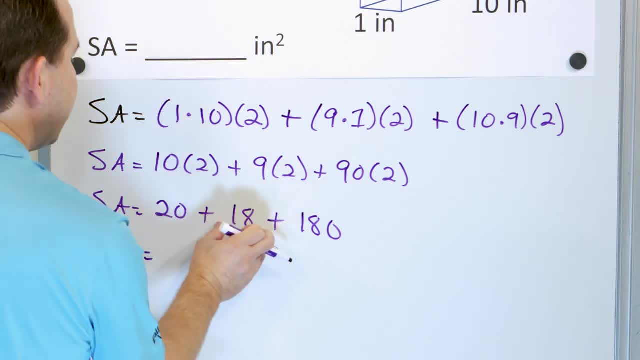 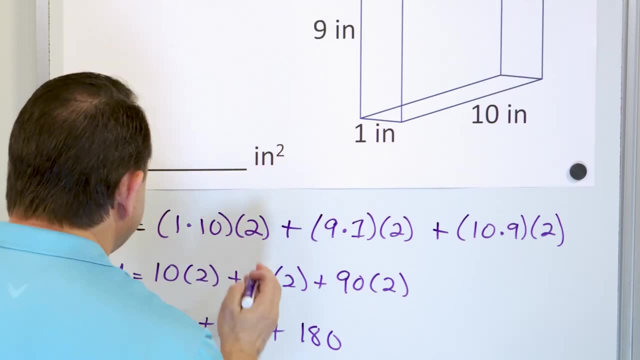 You can see that with the 180 and the 20,, that's 200.. 218 will give you a total of 218, and the units are square inches because I have inches everywhere, So square inches, So 218 is the final answer. 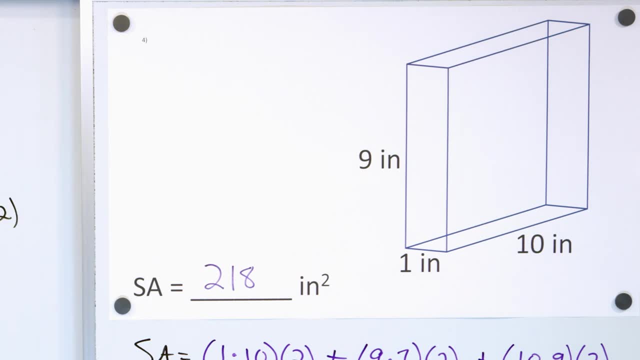 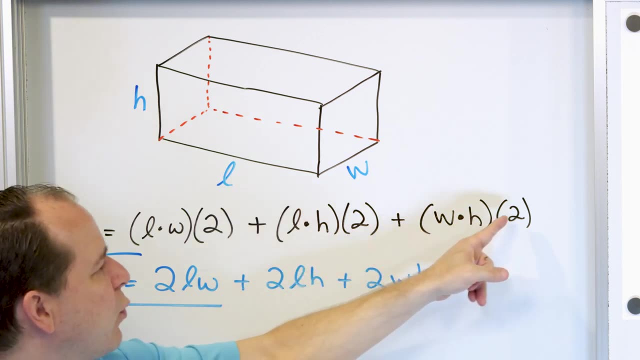 All right. So notice that when I started the lesson, I drew a picture, I put letters to illustrate the length and the width and the height of a rectangular prism And I showed you how we arrived at this equation down here. And this equation is what you will usually see in a class or in a book, or your teacher. 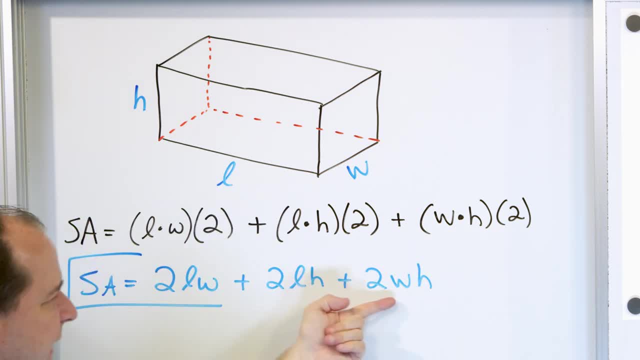 or somebody will say: use this, But I don't know about you. If you want to look at this, I get a little overwhelmed. There's so many letters. They're all in different positions. It's real easy to get confused. 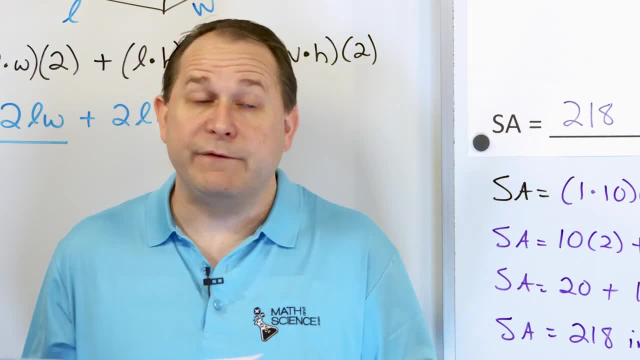 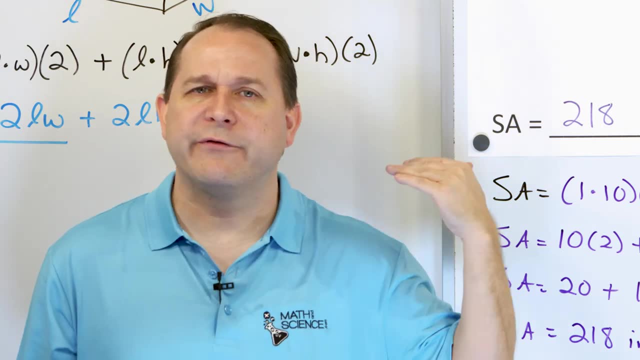 Is it LH or is it LW? It's very easy to get confused and to take the proper number and put it in the proper position And then, even when you get the answer, you don't really know what you're doing if you just follow it, because it's just a bunch of letters.